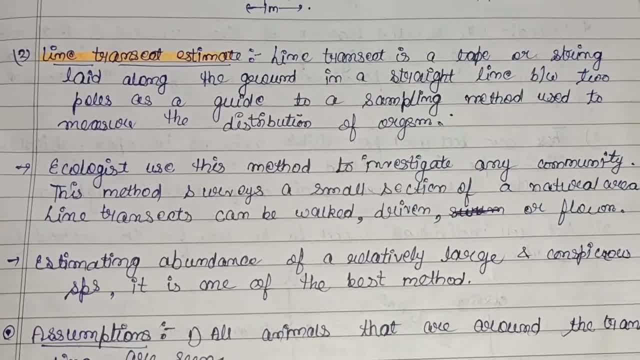 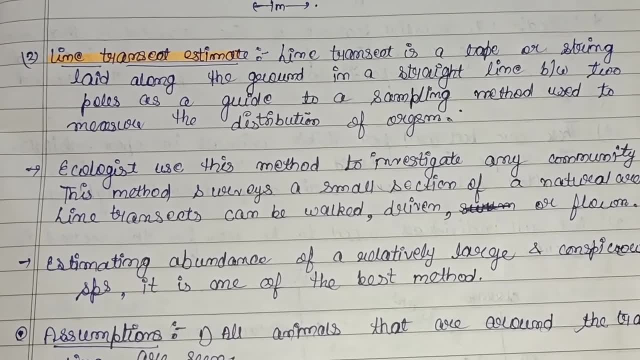 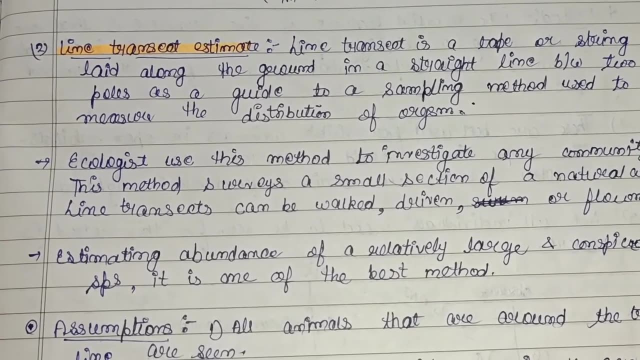 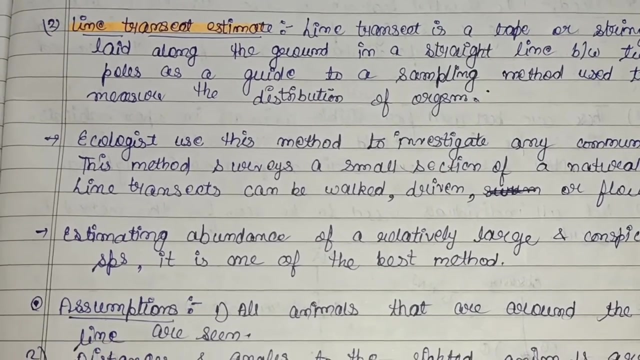 is very small. according to our raw material it is very small and therefore can be seen that the Ноx esp consolidates. the 인� Обный term is good task for this publication and can help in effective analysis of individual species. a view of identificationsw ie index of number of species, nearly 30.1 in this example. 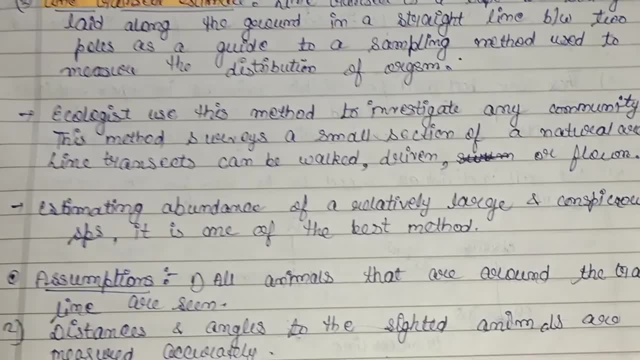 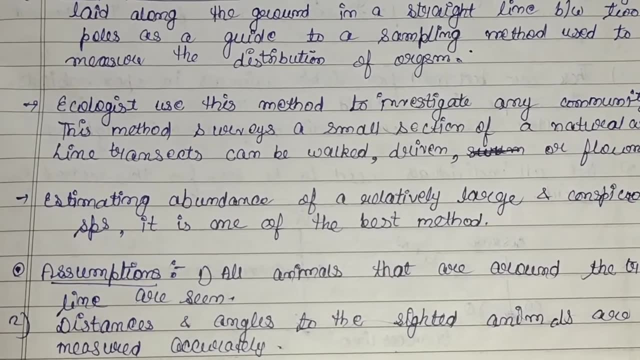 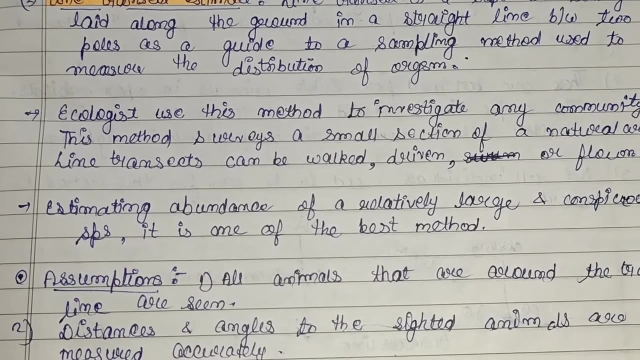 estimate of a relative large and conspicuous age ie sp comida. The first is that is all animals that are around the transect line are seen easily. Now the distance and the angles to the sighted animals are measured accurately, as this method involves various angles and the measurements, so that the measurements are accurate in nature. 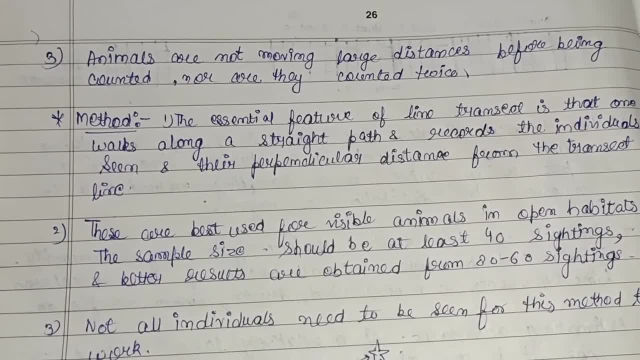 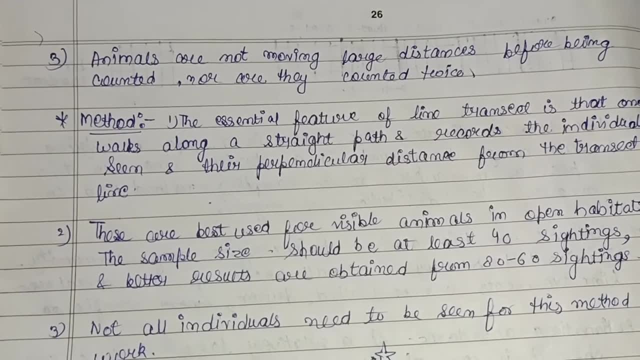 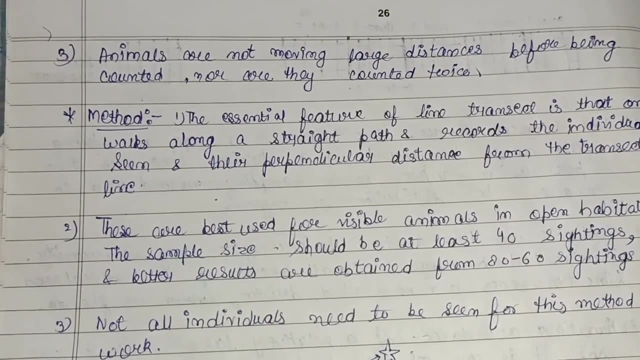 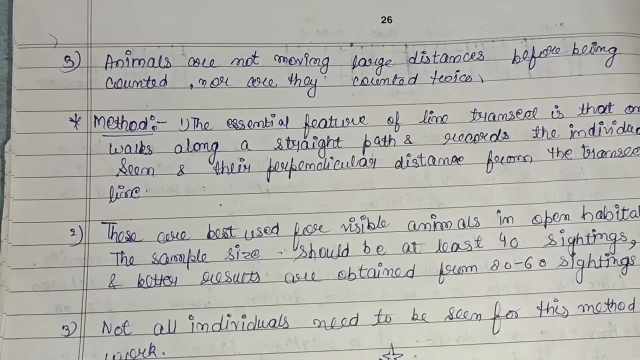 And also in this method animals are not moving large distances, that is, the strips are laid over large distance so that there are less chances of animal being moved to another habitat or another location. so before being counted, So all the animals are counted easily and nor are they counted twice, that is, there is no chance of count of a particular animal twice. 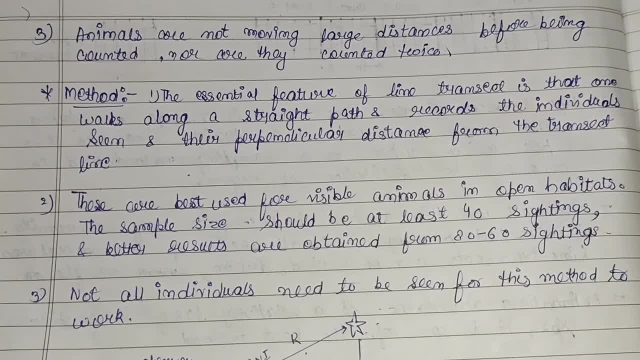 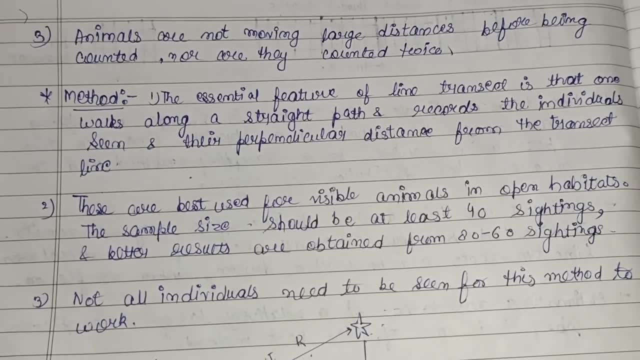 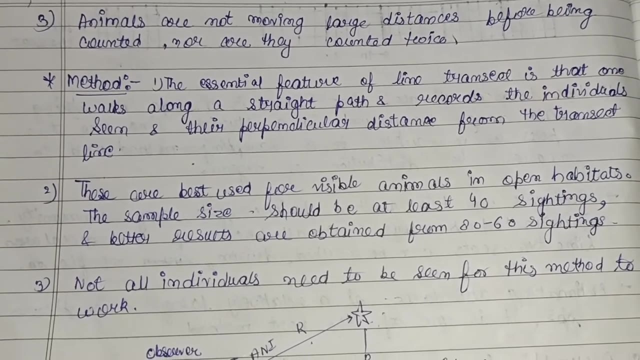 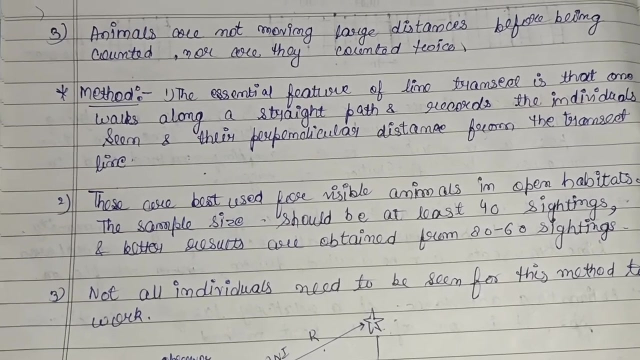 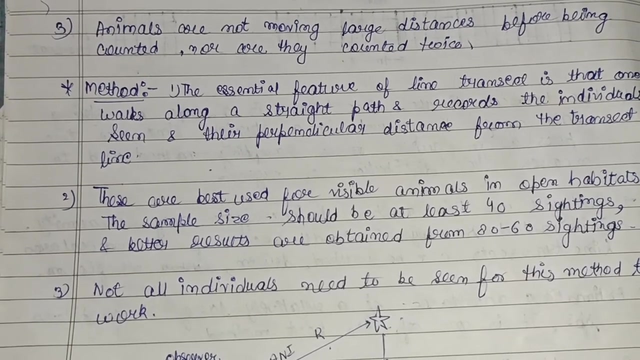 Now the method that is the Essential feature of the line transect is that one walks along a straight path and records the individuals that are seen, okay, and the perpendicular distance from the transect line, as we can see in the diagram later. So these are the best used for the visible animals in the open habitats, that is, basically the habitats which are not covered by dense forest or anything else, like the barriers, like rocks, etc. 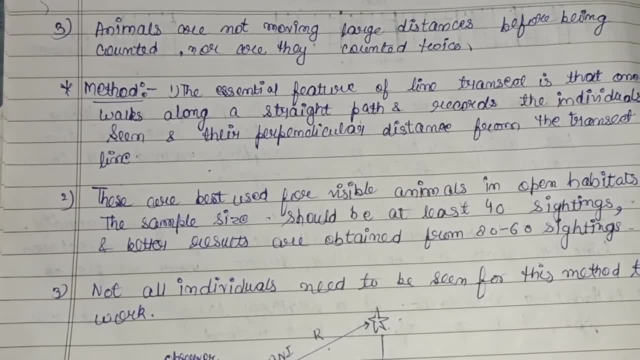 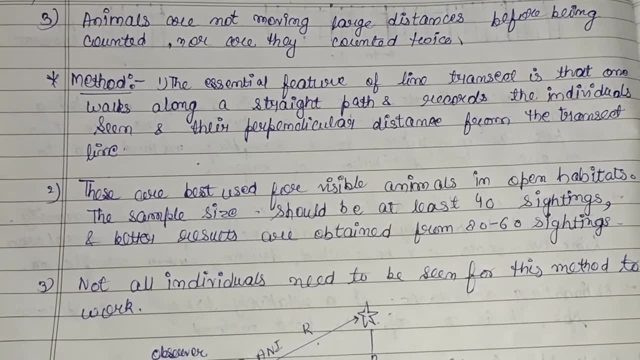 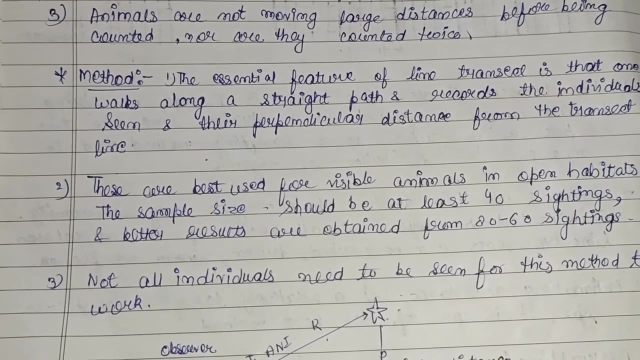 So that we can easily analyze or see the animals. to count, the sample site should be at least 40 sightings, that is, we should take over the 40 sightings and the for better results are obtained from 8 to 60 sightings from the ecologist or the observer. 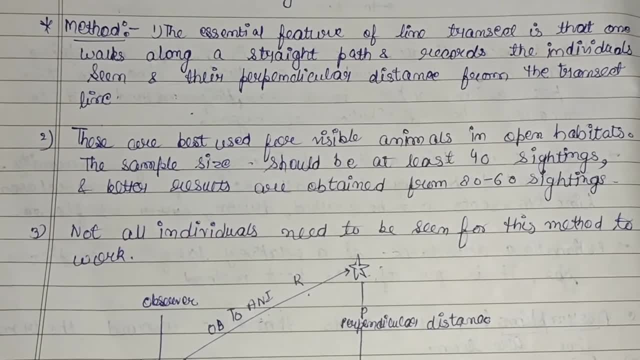 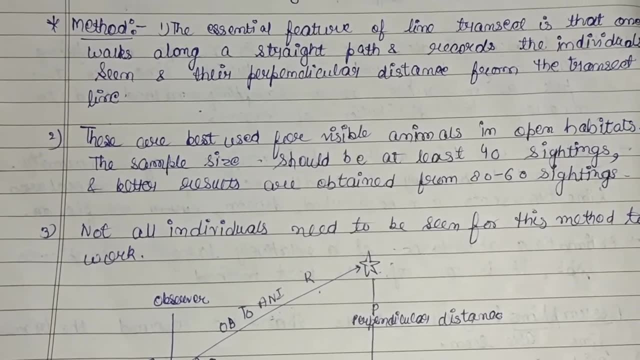 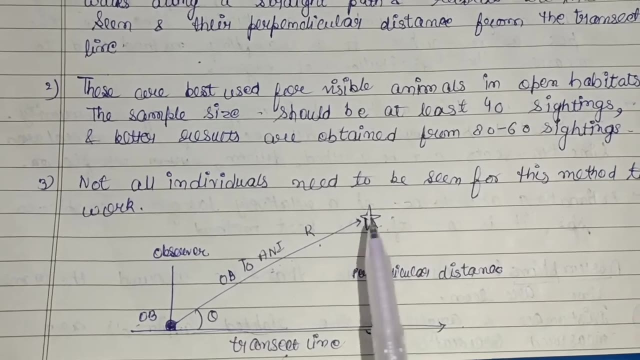 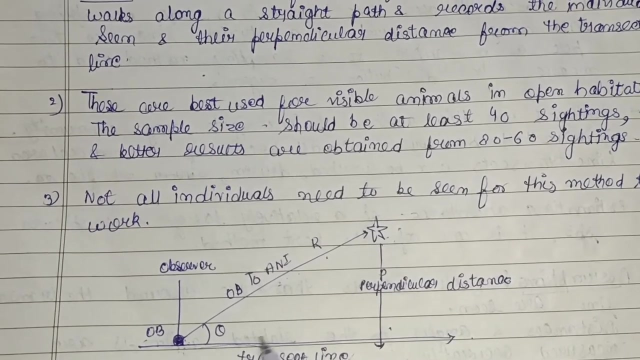 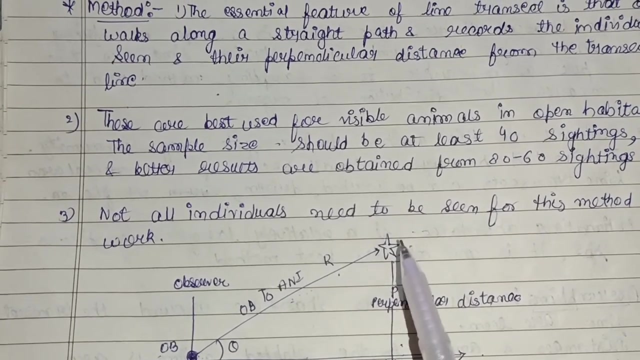 So not all individuals need to be seen for this method to work, that is, we have to count a certain species or the certain number of them so that the results are available. So this is a diagram. basically, this is the transect line that is late. and now this is the observer here to observe the species of the particular animals, and this is the perpendicular distance in which that observer moves. okay, and now this is the position of the observer to the targeted animals of a particular sighting. basically, 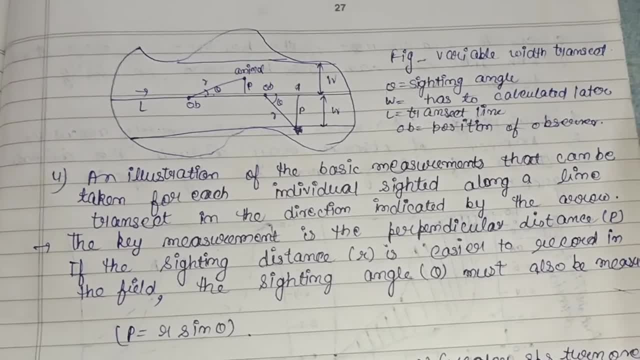 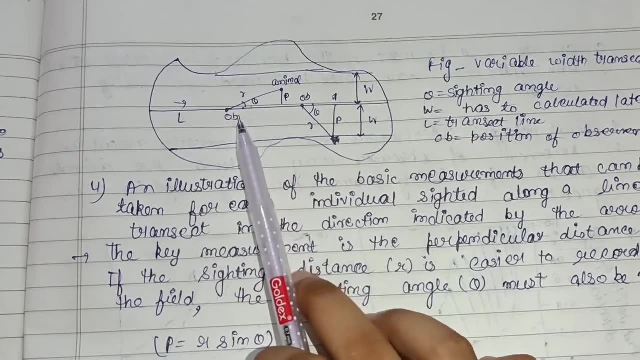 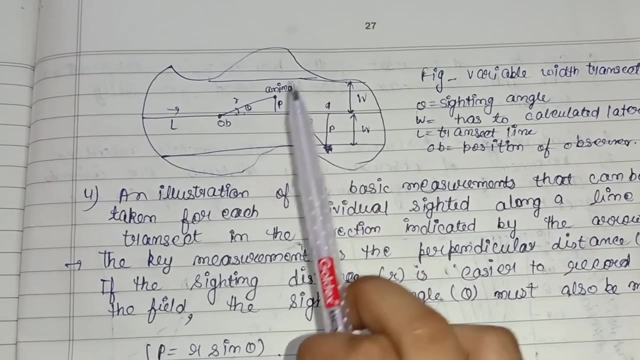 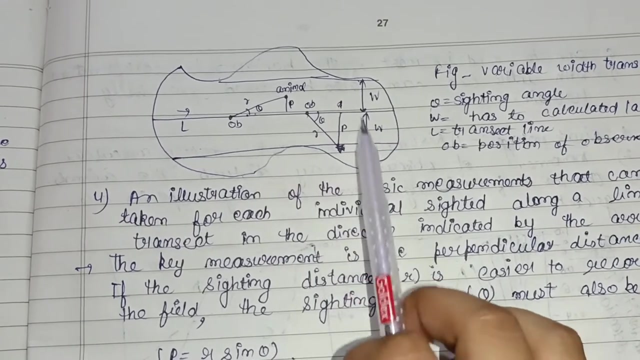 This is another diagram representing the variable width transect, that is, the. Here the transects are laid down representing the L: okay, observer is here. theta represents the sighting angle. W, that is has to be calculated later. okay, it has the animal. okay, that is being observed by the observer. the perpendicular distance that are laid along a particular transect line and OB represents the position of the observer. 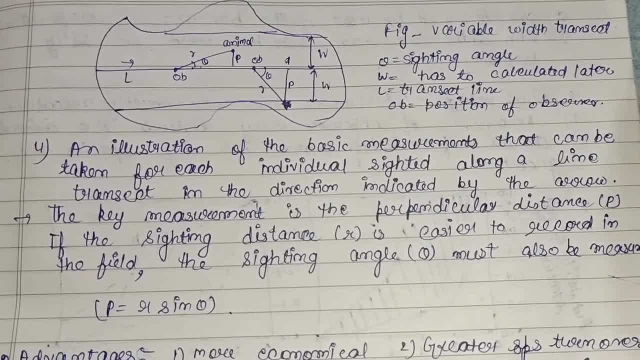 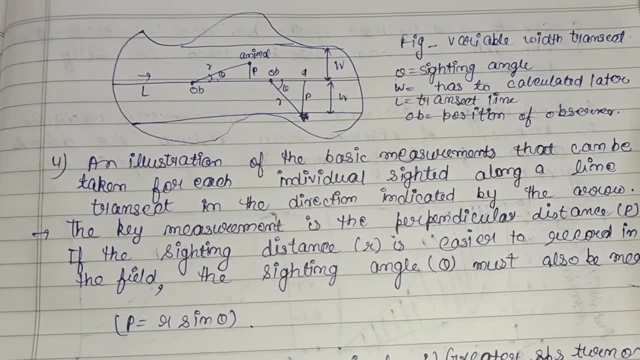 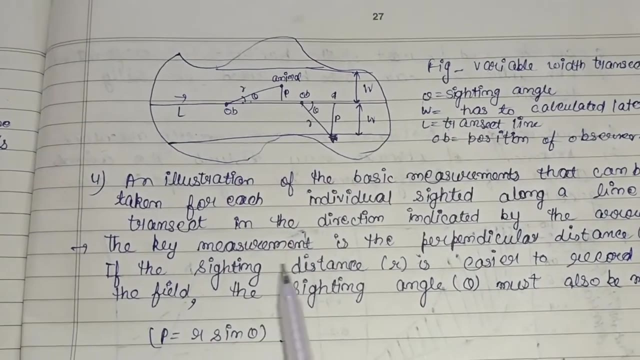 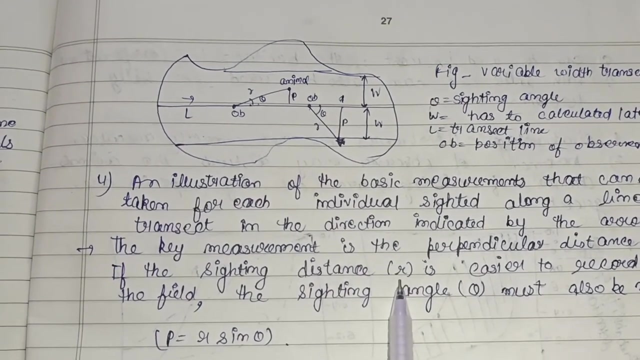 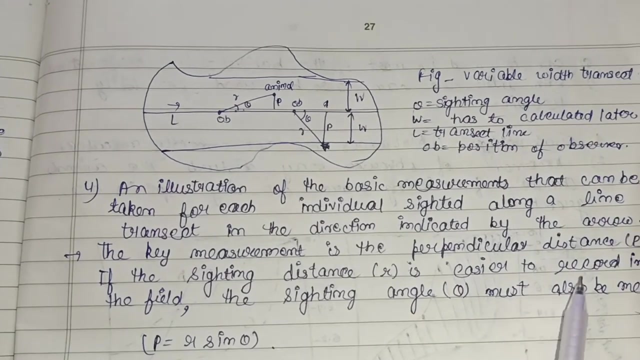 So this is an illustration of the basic measurements that can be taken for each individual That is sighted along a line and transect in the direction that is indicated by the arrow. so this is the direction that is indicated by a particular arrow. so the key measurement is the perpendicular distance, P, that is, we have denoted here. if the sighting distance R, that is, the R that is setting distance between the observer to the particular animal sighted animal, is easier to record in the field, the sighting angle, theta, must be. 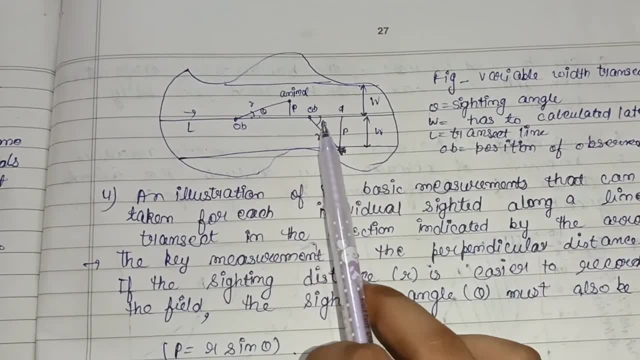 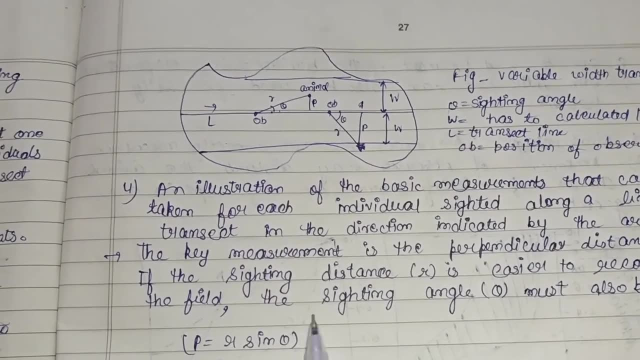 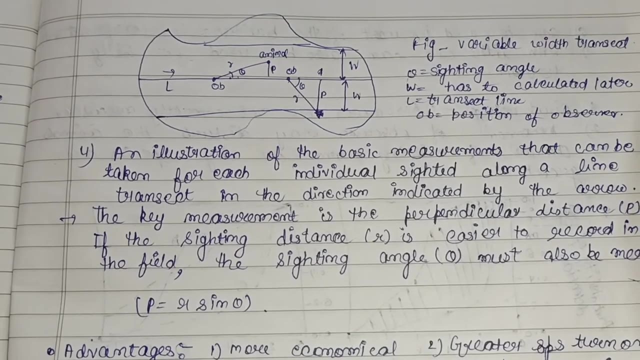 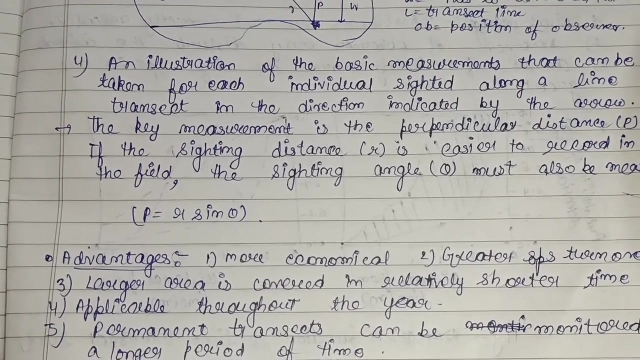 Measure, that is for calculating the R, we must know the angle, that is the theta, that is the sighting angle. so the formula here is: P is equal to R sine theta, that is For measuring the perpendicular distance. so this is the overall method for the line transect estimate method. now the advantages. so it is more economical, that is, it is cheap and easier. affordable, we can say, greater species turnover is seen in that case. that is mostly. 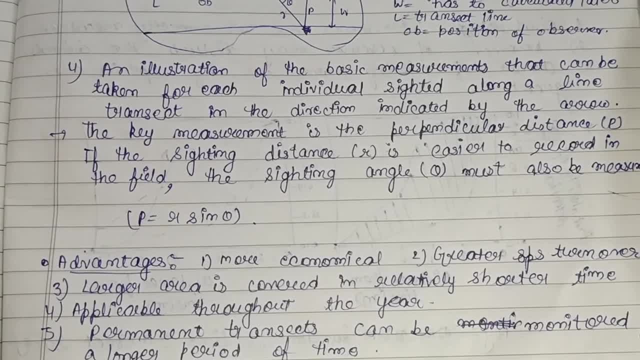 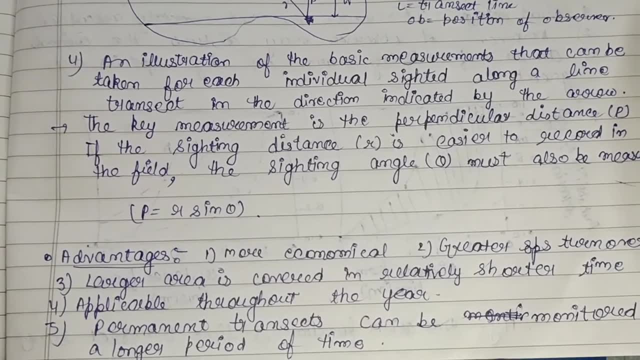 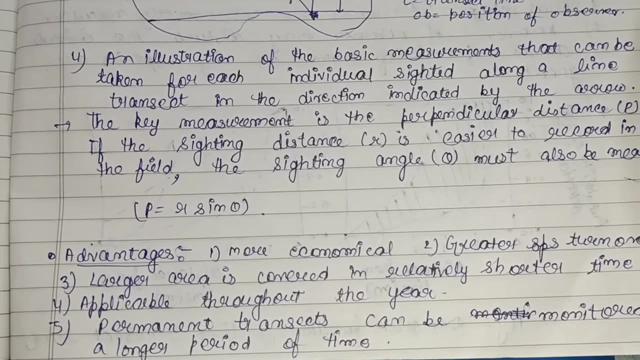 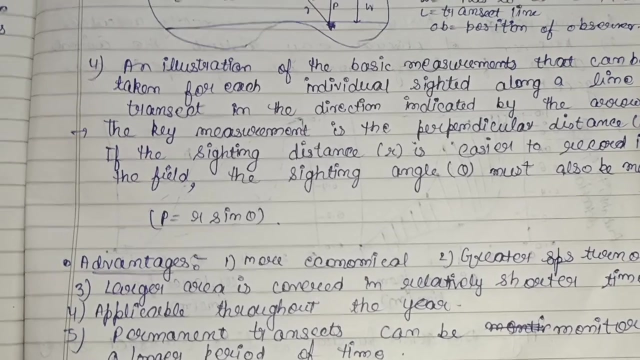 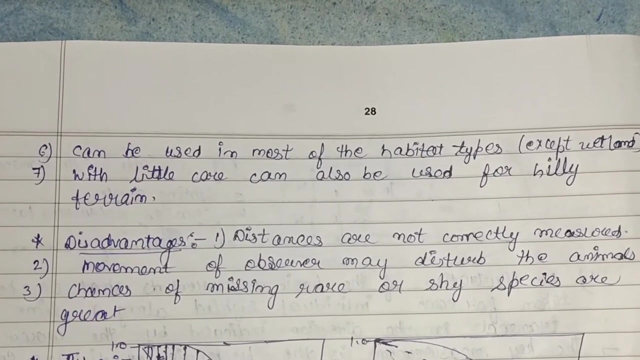 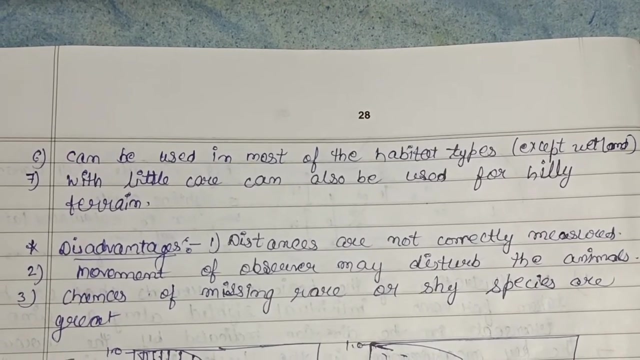 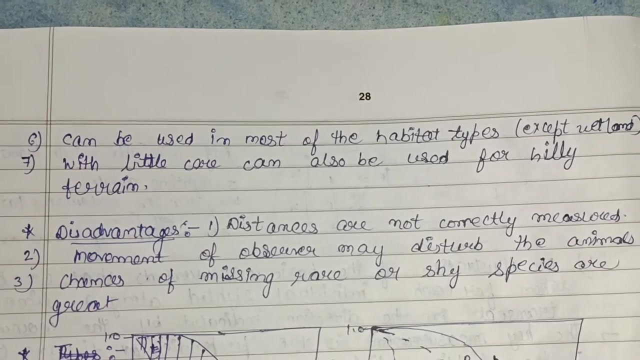 Release the that they can be observed over a longer period of time. Ten Here Are Lines: The Also. another advantage is that is they can be used in most of the habitat types, whether it is aquatic or the terrestrial habitat, except their wetlands. Now, with little care, it can also be used for hilly terrains also. 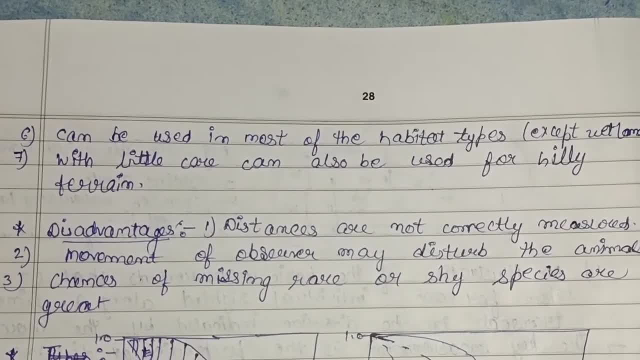 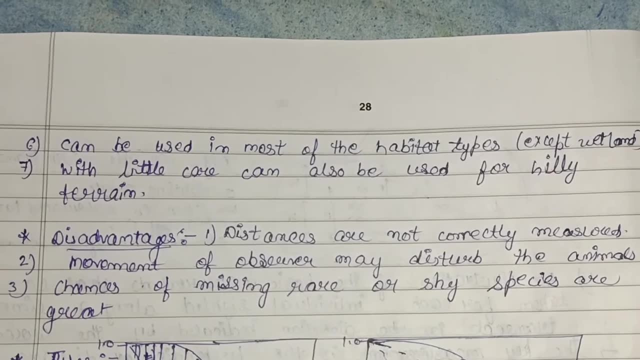 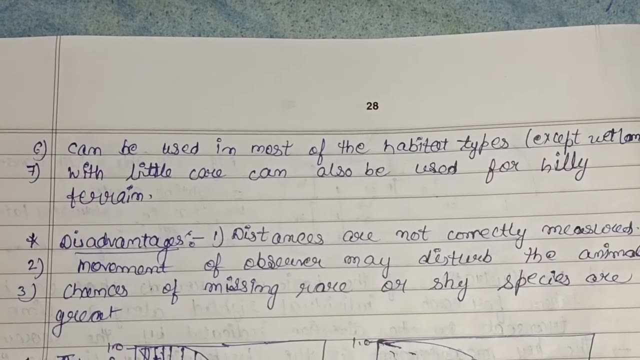 So now the disadvantages that it possess. so distances are not correctly measured, that is, there should not be a complete accuracy in that. Movement of observer may also disturb the animals so that they are not able to cross the line. and in case of line transact method, only those species are counted which cross the or touch the transact line. 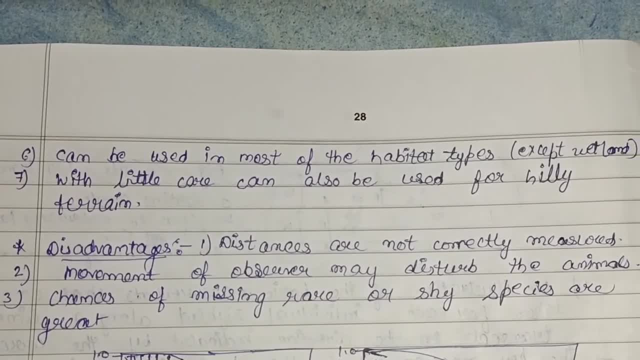 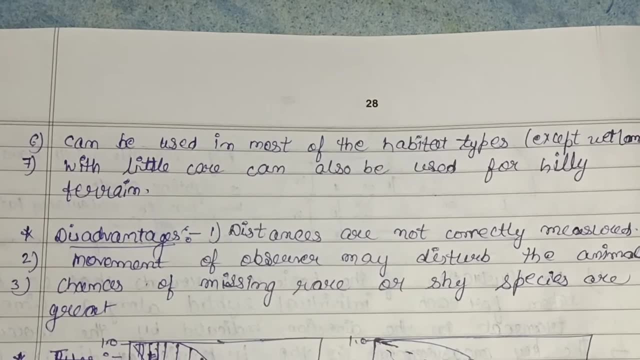 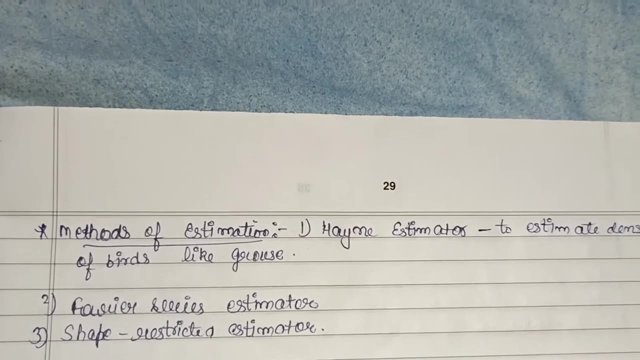 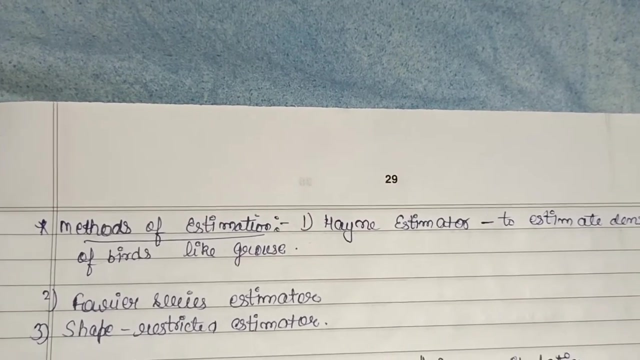 So the chances of them missing the rear or the shy species are great because as they are not able to touch that particular line or enter that particular line. So this is the disadvantage. now there are also various methods of the estimation of the animal population, like the Heine estimation to estimate the densities of the bird species, like the grouse, then the Fourier series estimator and also the shape restricted estimator. 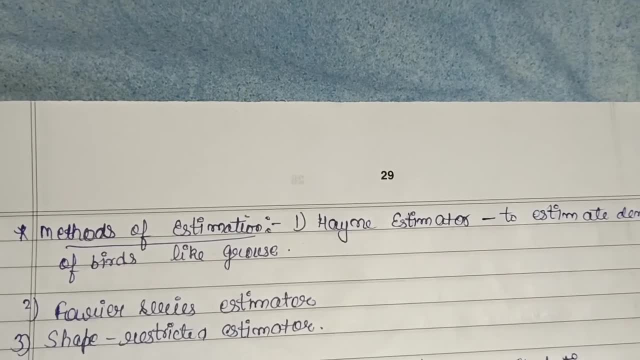 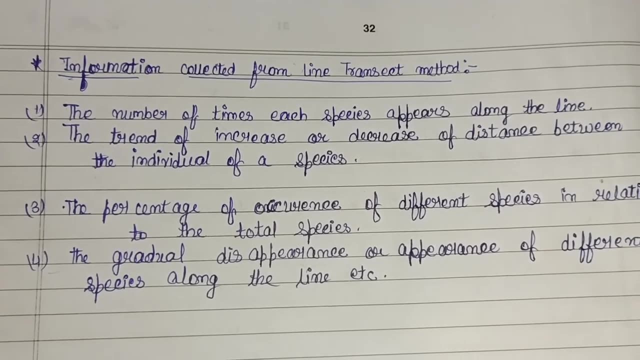 The further details are not required as per the syllabus of the UG or the PG students. Now, the information that is required for the UG or the PG students is that they should not be used for hunting. So this is the percentage of the species collected from the line. transact method is like that. that is, first, is the number of the times each species appears along the line is counted here. 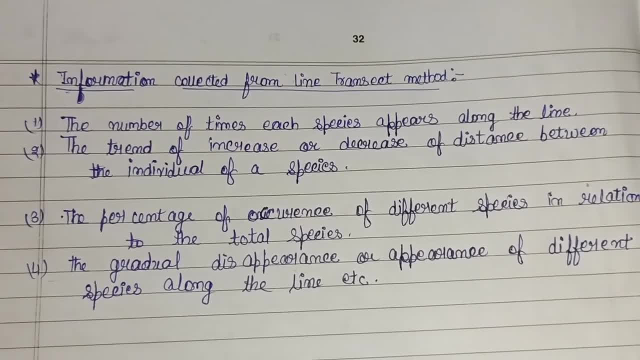 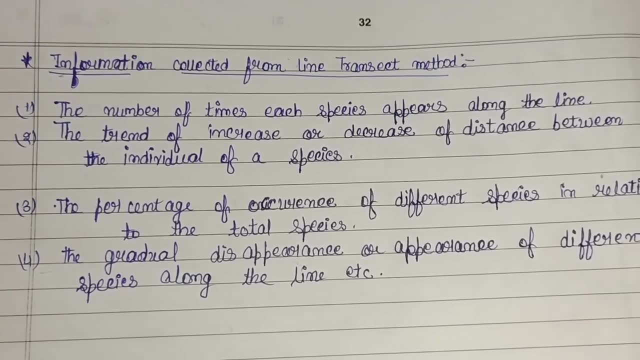 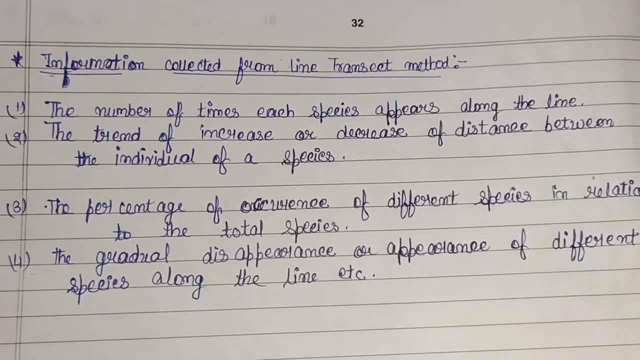 then the trend of the increase or decrease of a distance between the individual of a species is also observed. Then the trend of the increase or decrease of a distance between the individual of a species is also observed. The percentage of the occurrence of different species in a relation to total species, that is in case as some species, members of some species, got away from the particular total species. the number of times that each species appear is well known. 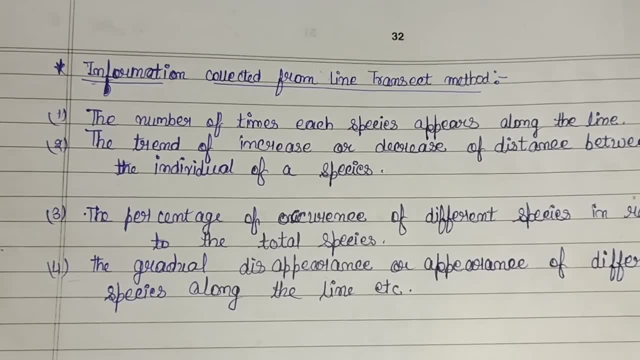 Data analysis. also, mezac's are taken into account Forever on depict the differences of a species. and if sex keeps the same, or no sex per species, then the result of the- Well, incom Minne the the- Here, let us observe the number of species have to be counted as per case.